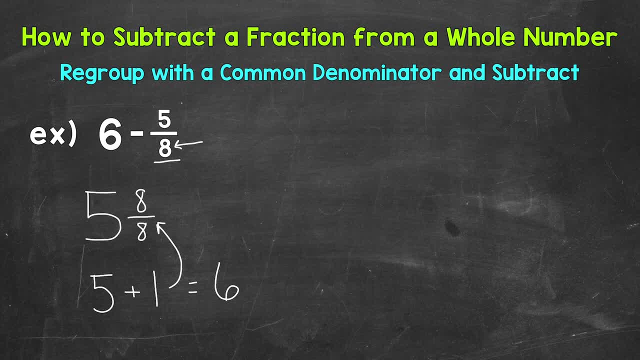 Now we can subtract. So I'm going to come to the side here and write our mixed number: So 5 and 8, eighths, and again that's equivalent to 6. And we are subtracting, Subtracting 5 eighths. 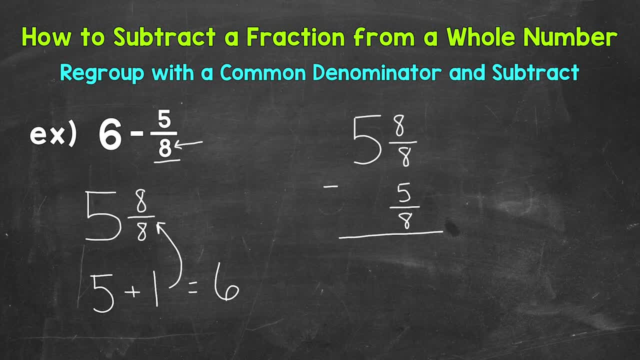 So I can line up my fractions and now subtract, So I can do 8 eighths minus 5 eighths, which gives us 3 eighths, And then we can take a look at the whole number. So we have 5 minus, and then we don't have a whole number there, so we just drop our 5 down. 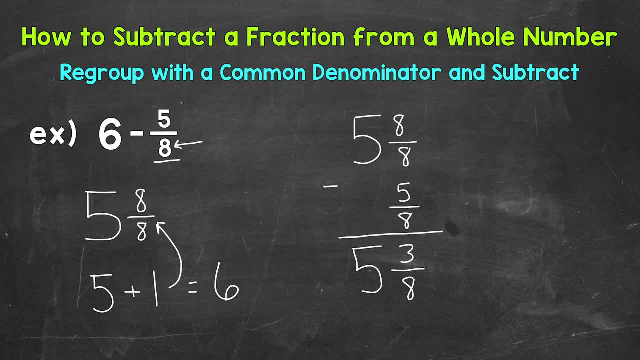 And we get an answer of 5 and 3 eighths. We can always look to see if we can simplify the fractional Part of a mixed number. 3 eighths is in simplest form. The only common factor between 3 and 8 is 1.. 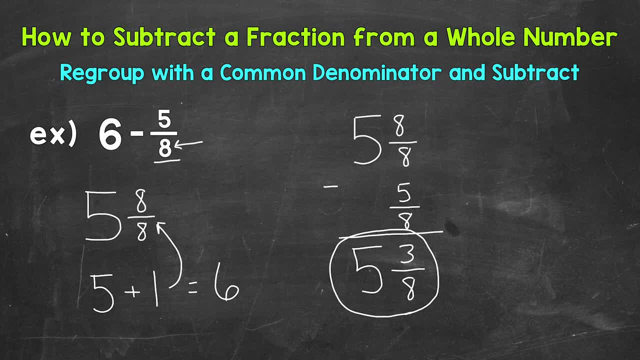 So this is done, and in simplest form. Now one more thing I do want to mention. You can write this horizontally, meaning side to side, if you prefer that way. So 5 and 8 eighths minus 5 eighths. 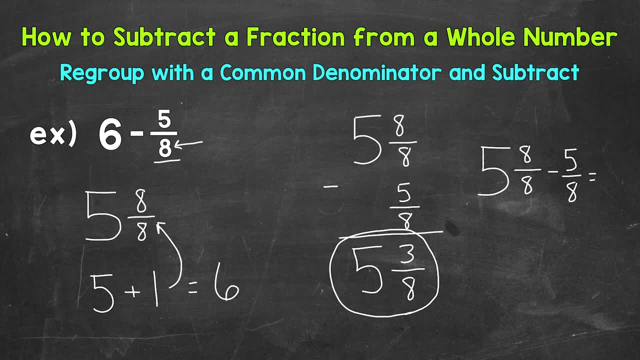 And that gives us. Well, subtract the fractions, we get the same thing: 3 and 8 eighths, 3 eighths for our fractions, and then we have 5 wholes, So 5 and 3 eighths horizontally as well. 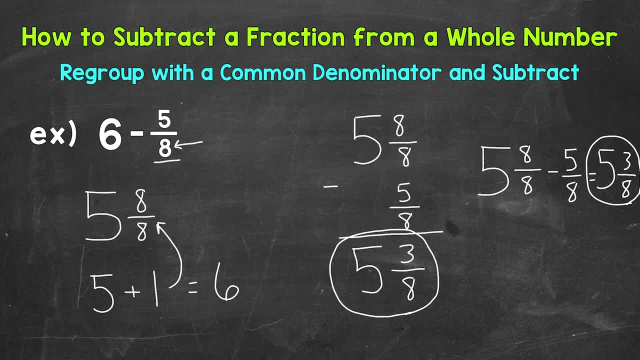 So there you have it. There's how you subtract a fraction from a whole number, Regroup or change that whole number to a mixed number where the fractional part of the mixed number equals 1. Then we can subtract the fractions and take a look at the whole number to get our final answer. 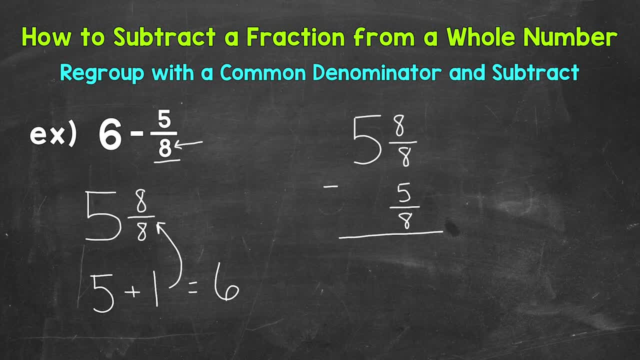 So I can line up my fractions and now subtract, So I can do 8 eighths minus 5 eighths, which gives us 3 eighths, And then we can take a look at the whole number. So we have 5 minus, and then we don't have a whole number there, so we just drop our 5 down. 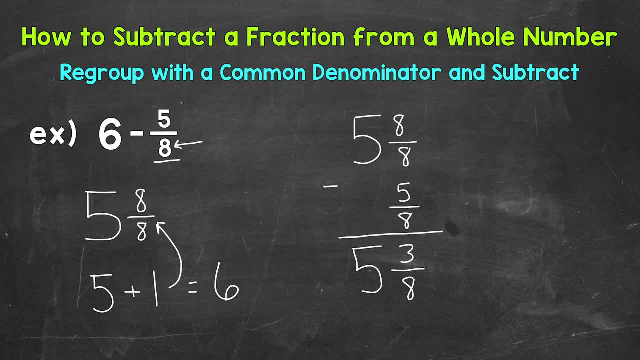 And we get an answer of 5 and 3 eighths. We can always look to see if we can simplify the fractional Part of a mixed number. 3 eighths is in simplest form. The only common factor between 3 and 8 is 1.. 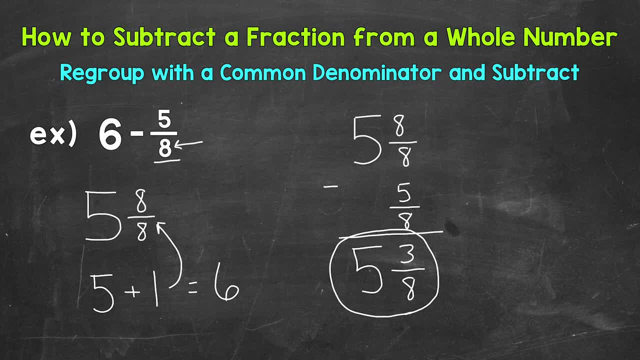 So this is done, and in simplest form. Now one more thing I do want to mention. You can write this horizontally, meaning side to side, if you prefer that way. So 5 and 8 eighths minus 5 eighths. 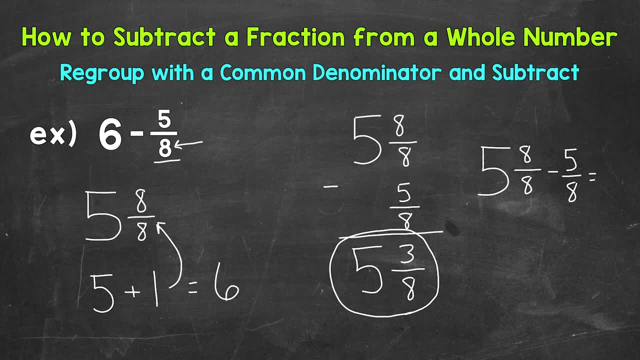 And that gives us. Well, subtract the fractions, we get the same thing: 3 and 8 eighths, 3 eighths for our fractions, and then we have 5 wholes, So 5 and 3 eighths horizontally as well. 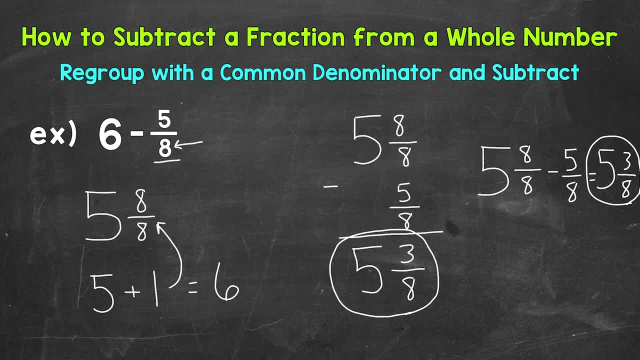 So there you have it. There's how you subtract a fraction from a whole number, Regroup or change that whole number to a mixed number where the fractional part of the mixed number equals 1. Then we can subtract the fractions and take a look at the whole number to get our final answer. 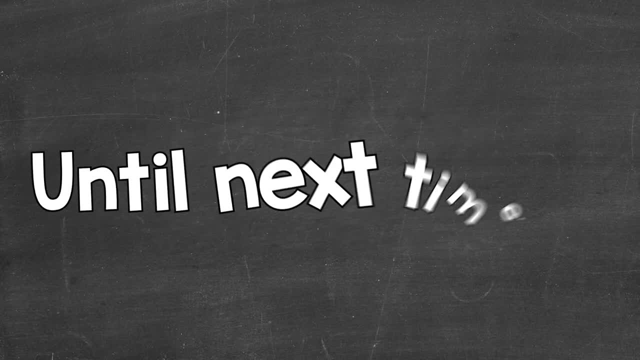 I hope that helped. Thanks so much for watching. Until next time, peace. 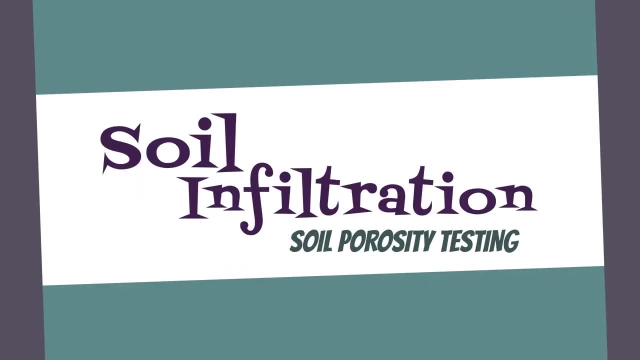 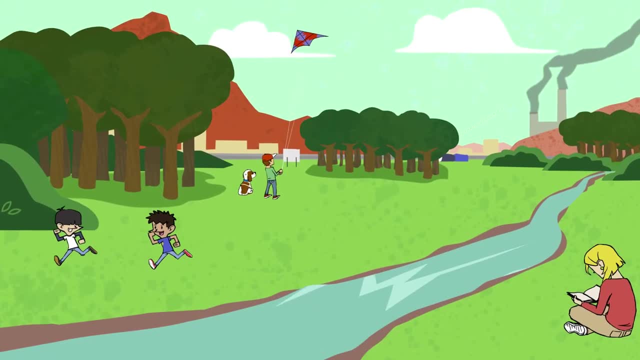 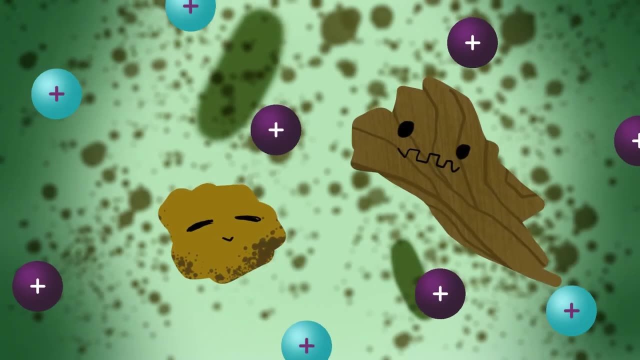 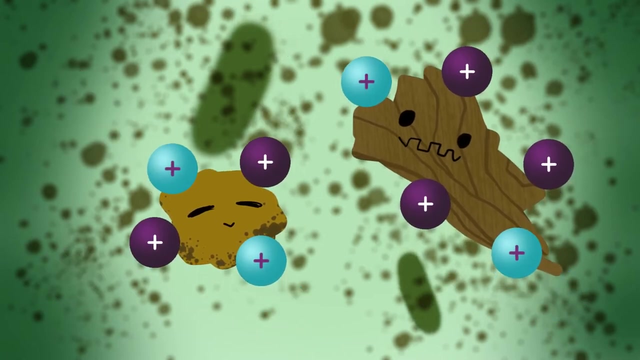 Streams in natural areas are important to our communities. People and their pets walk near them. children play in them. Unfortunately, when streams are near industrial areas, there's sometimes accidental contamination from heavy metals or other chemicals. Contaminants can hold onto or sorb the clay and organic matter that is suspended in muddy-looking waters.